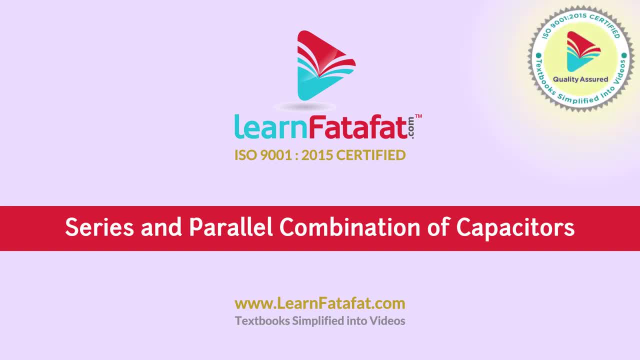 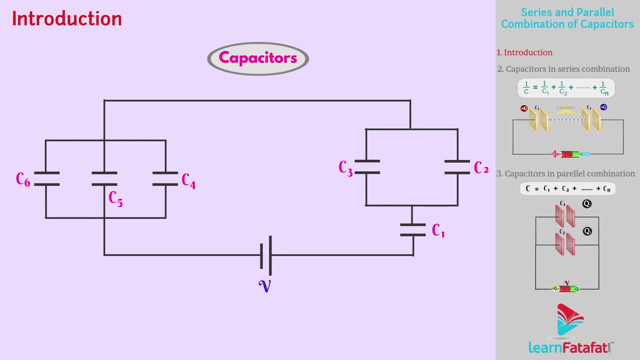 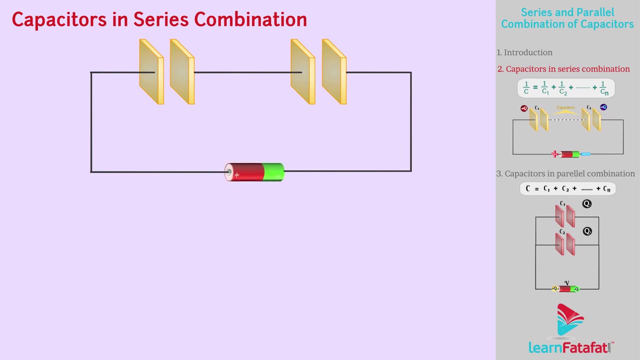 These students. capacitors can also be combined to form various arrangements. The simplest two of them are series combination and parallel combination. In case of capacitors in series combination, right plate of one capacitor is connected to left plate of other capacitor and the end plates of the arrangement is connected to battery. 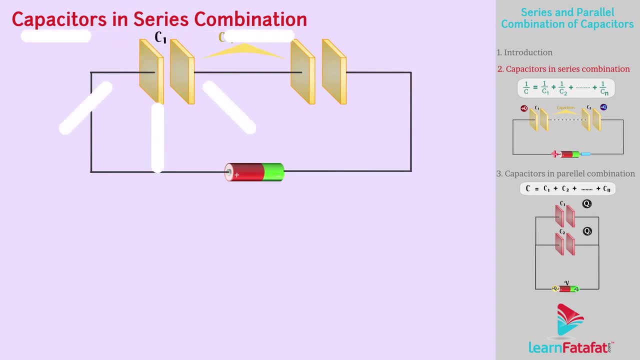 Suppose there are two capacitors, C1 and C2 are connected in series, Left plate of C1 connected to positive terminal of battery and right plate of C2 connected to negative terminal of battery. The battery supplies charge plus Q to left plate of C1. 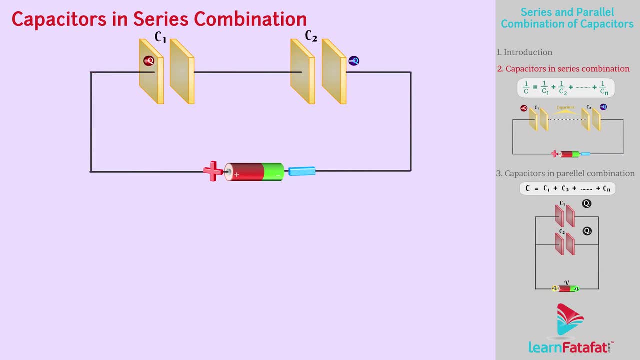 and minus Q to right plate of C2 respectively, Due to which there is minus Q charge on right plate of C1 and plus Q charge on left plate of C2.. Plate with plus Q charge produce electric field that tend to bring opposite charge on right plate. 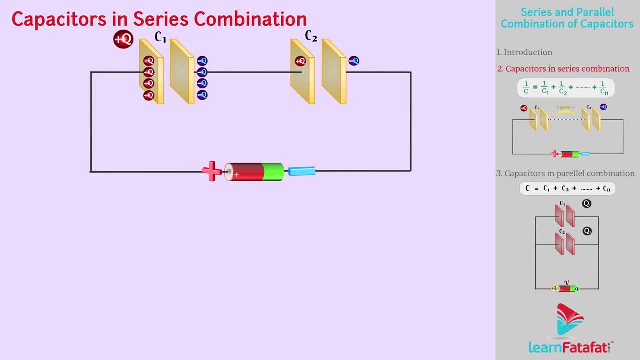 Similarly negative electric field of minus Q tend to bring plus Q on its left plate, which is done by transfer of charges through the conductor. This means that both capacitors carry equal charge, that is Q. Now, as the capacitors are connected in series, 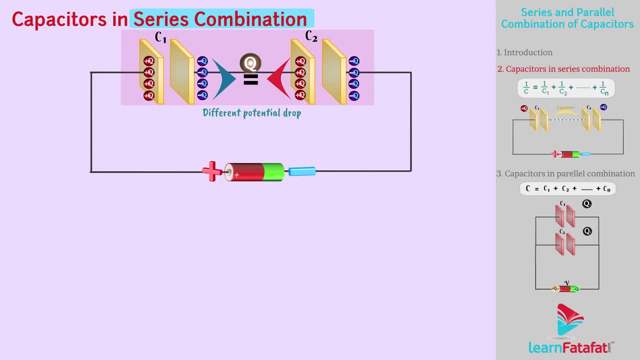 there must be different potential drop across each capacitor. So if V is supply voltage, V1 is potential drop across C1 and V2 is potential drop across C2, then V equals to V1 plus V2.. But for C1, we have: V1 equals to Q by C1. 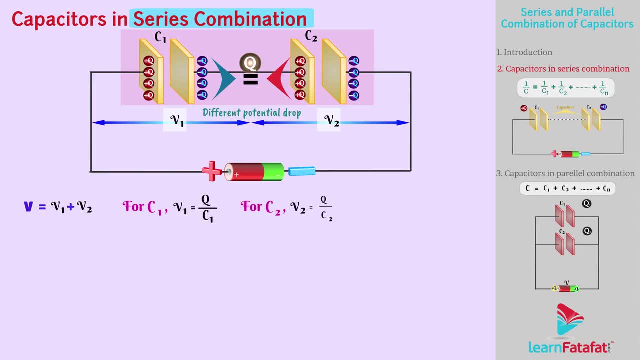 and for C2, we have: V2 equals to Q by C2. So V equals to Q by C1 plus Q by C2.. So V by Q equals to 1 upon C1 plus 1 upon C2.. Let's call this as equation number 1.. 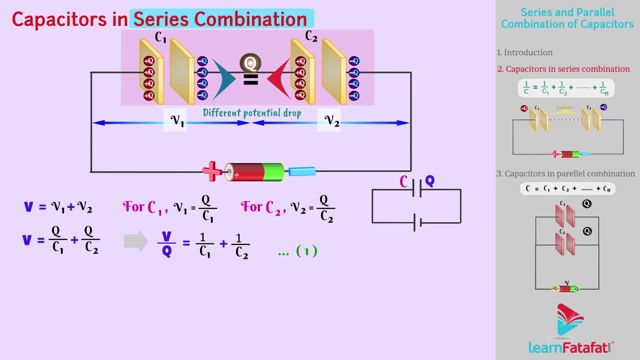 If we think an equivalent capacitor having charge Q and potential difference V, then the capacitance C will be: C equals to Q by V. Let's call this as equation number 2.. Now, comparing 1 and 2, we can write: 1 upon C equals to 1 upon C1 plus 1 upon C2.. 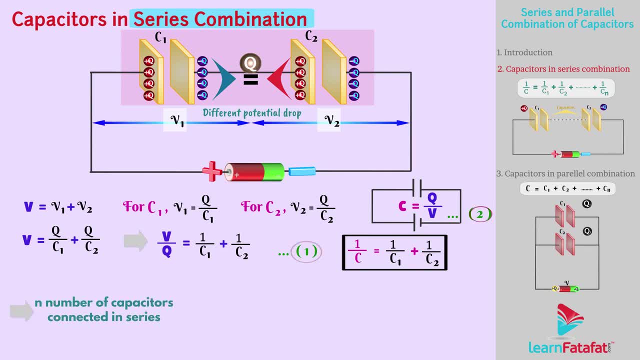 If there are n number of capacitors connected in series, then with similar analysis we can find that 1 upon C equals to 1 upon C1, plus 1 upon C2 up to 1 upon Cn. This is the equivalent capacitance for series combination. 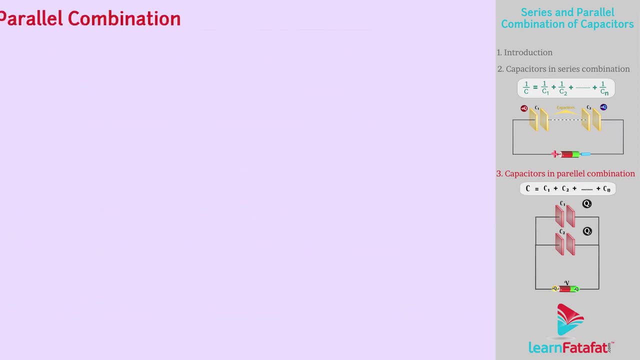 Let us try to find equivalence capacitor of capacitors in parallel combination. Suppose C1 and C2 are connected in parallel. then the potential difference across each capacitor will be equal to supply voltage. However, the charges differ. That is, the capacitor C1 holds charge Q1. 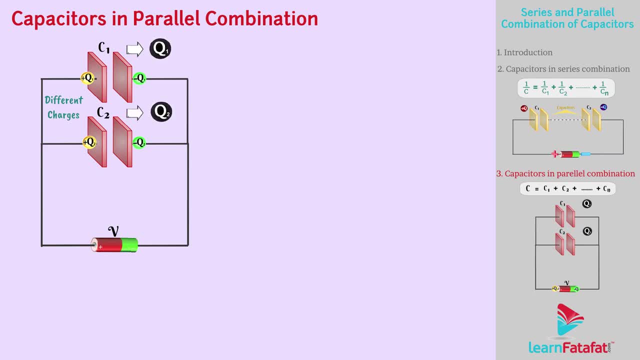 and capacitor C2 holds charge Q2, where Q1 equals to C1 into V and Q2 equals to C2 into V. If we imagine an equivalent capacitor having potential difference V across it and carrying charge Q, then we can write: Q equals to Q1 plus Q2, or. 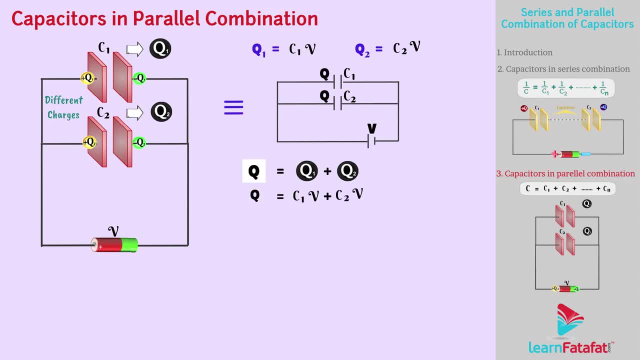 Q equals to C1, V plus C2 into V, or Q by V equals to C1 plus C2.. But we know that Q by V equals to C, which is equal to capacitance of equivalent capacitor. Therefore C equals to C1 plus C2..